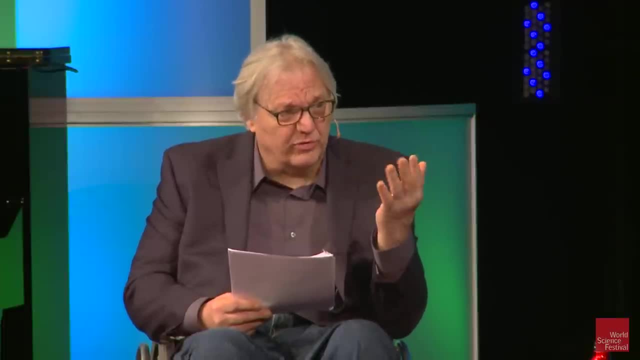 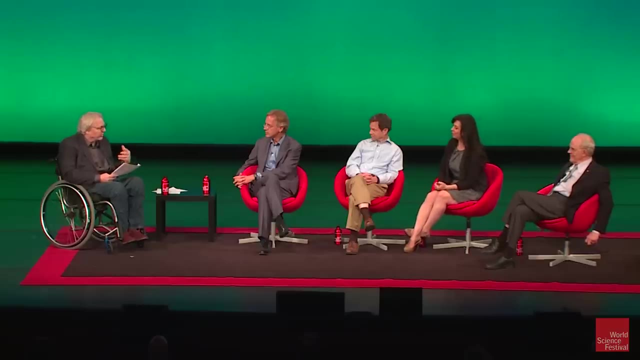 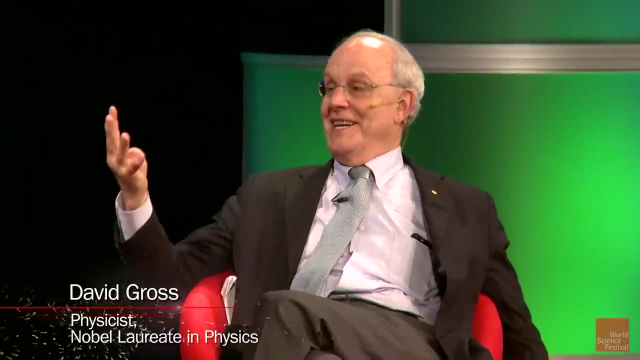 David Gross, we've got strong nuclear force, weak nuclear force, electromagnetic force and gravitational force right now. right? Is that a symmetric system, or is there an asymmetry there that forces us to look for something else or other things? Well, the fact that you had four names is obviously asymmetric and it's like four pieces of a jigsaw puzzle. 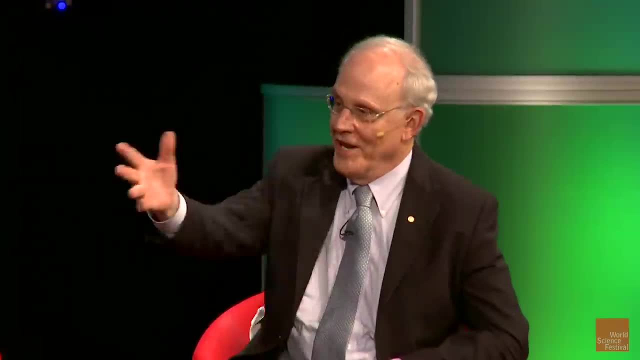 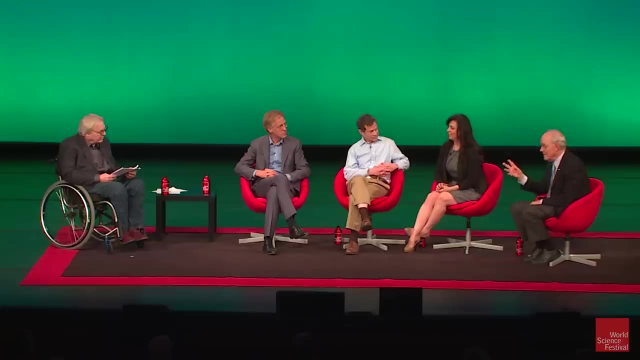 If I give you four pieces of a jigsaw puzzle, or 40, and you put them together, most likely I didn't give you all the pieces and there were a few holes. These pieces actually fit together and that was evident 30 years ago from the beginning. 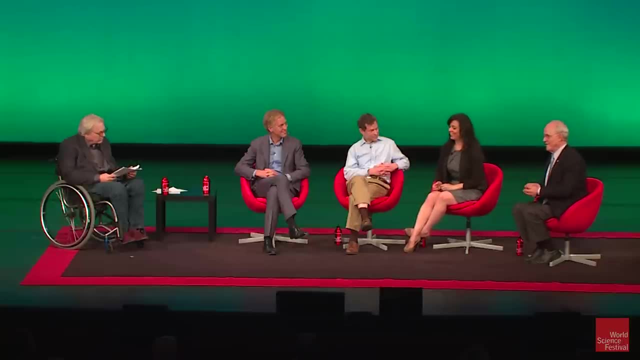 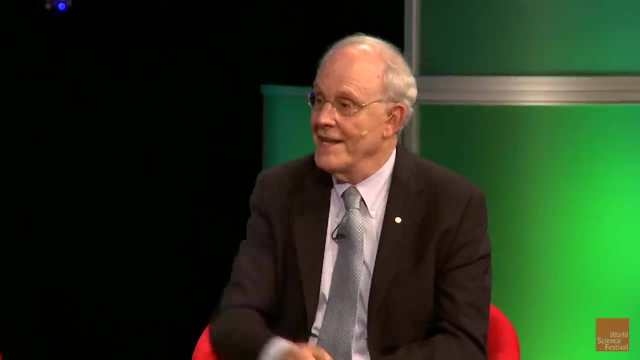 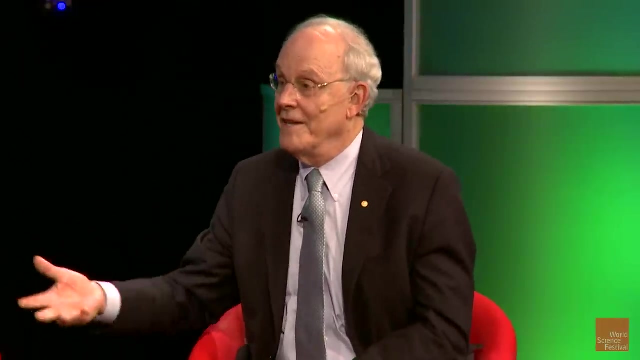 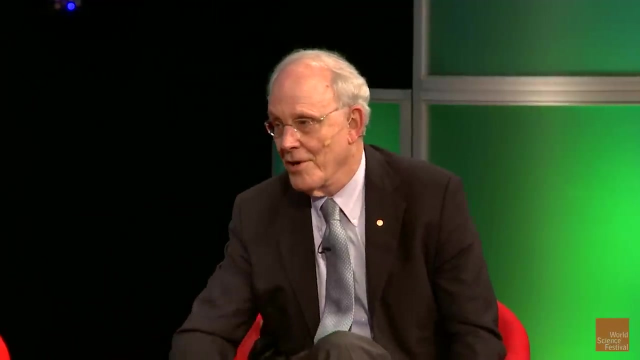 Three of the four, Three of the four, fit together beautifully into a sort of an obvious jigsaw puzzle. People then extrapolated that and discovered that if you really could look very deeply inside matter, even gravity fits into the picture. naturally, That's what has spurred an attempt for 30 years and more to try to unify all the forces. Unification is a standard goal of physics. It's been very successful. Newton unified apples and planets. They have the same motion, same cause for their motion, Although no one was asking him to unify apples and planets. It's a strategy. We've learned that it works. If you understand gravity, it acts on apples. It acts on apples and planets. Maxwell unified electricity and magnetism. Particle physics so far has unified quite a bit of the forces. But a unified force is simpler, more symmetric, more explanatory. So that's been a goal. 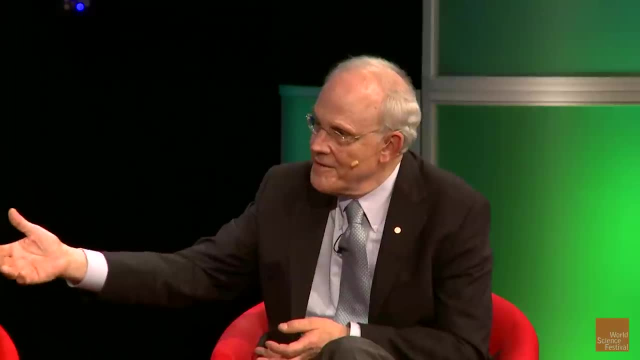 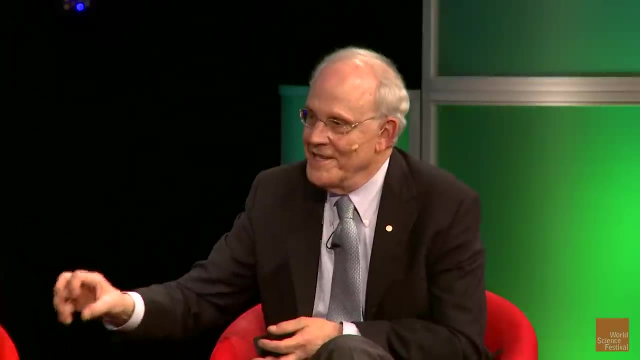 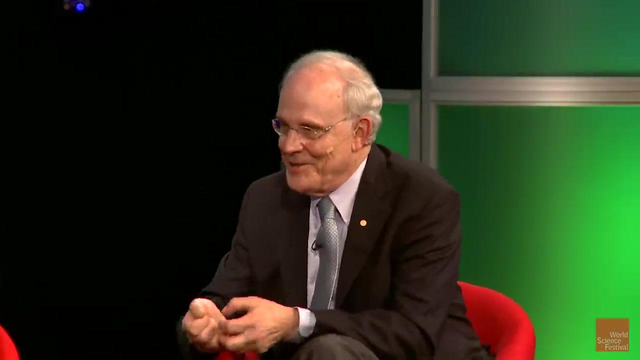 What about the fifth force that was announced in the last couple of weeks? The Higgs is kind of like a fifth force- The Higgs particle and its dynamics- That too would fit in the same picture. So there's overwhelming theoretical evidence or clues from nature and our understanding that unification should occur. 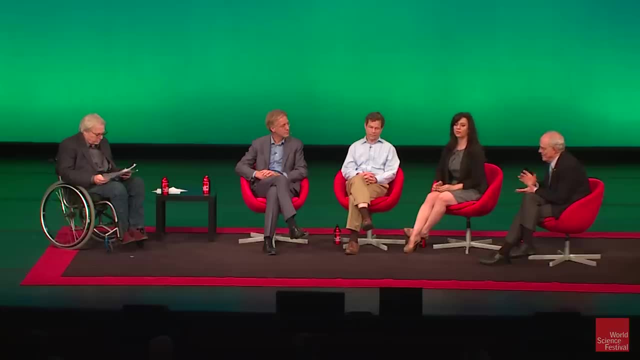 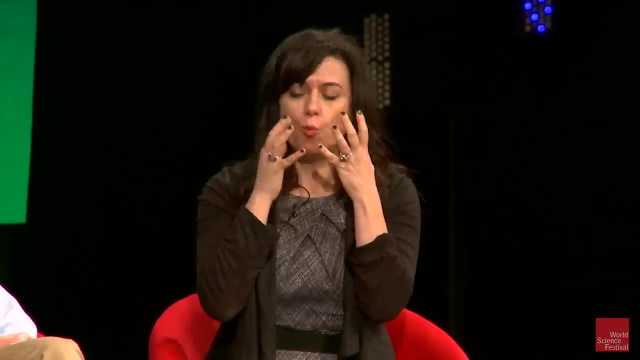 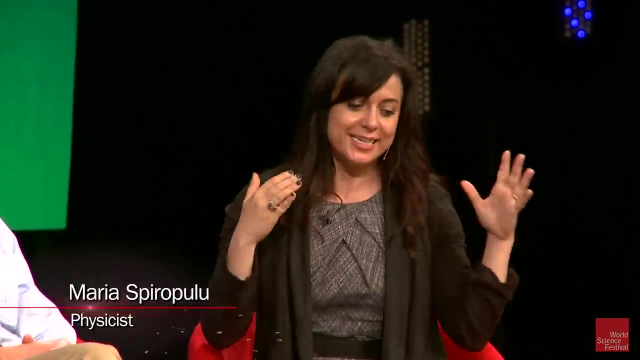 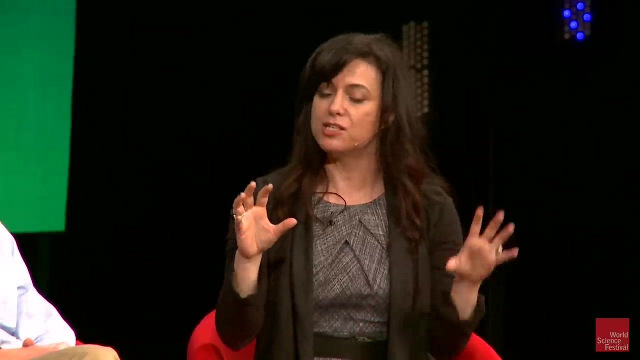 But how it occurs we still don't know. This is really the complete wanting the beauty and wanting the simplicity. It may be that it's not like that. This is a guiding principle from what we have seen, But it may be that this puzzle with gravity is not going to come together. 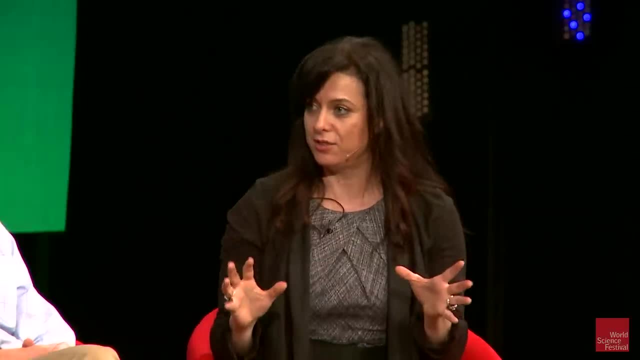 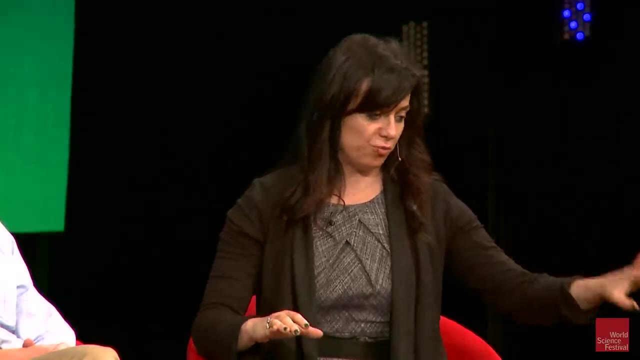 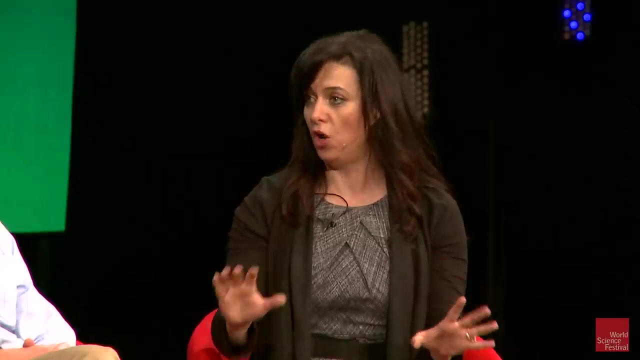 with the other three forces in our grand unified dream, let's say So. I think we need to keep things in perspective And because gravity connects with the cosmological constant and the dark matter problem, we kind of need to hold tight on how this picture evolves. 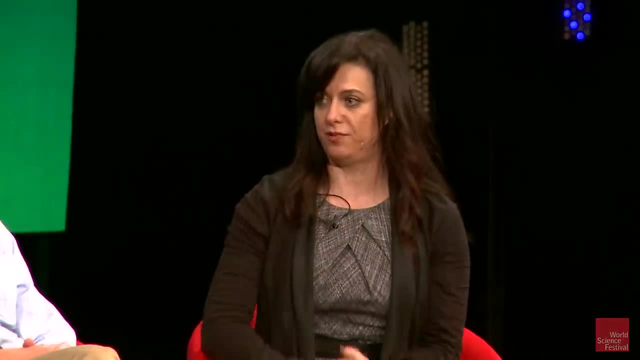 with all the forces and with the grand unified theory. Subtitles by Subtitle Workshop.